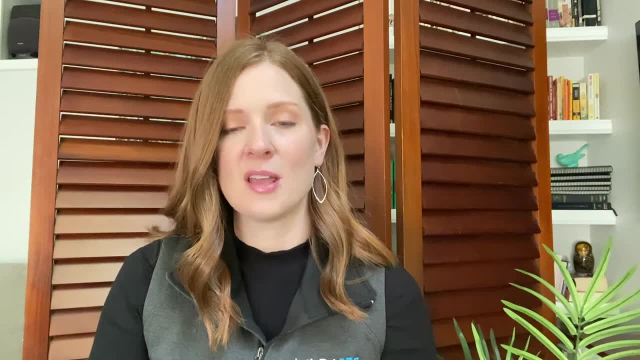 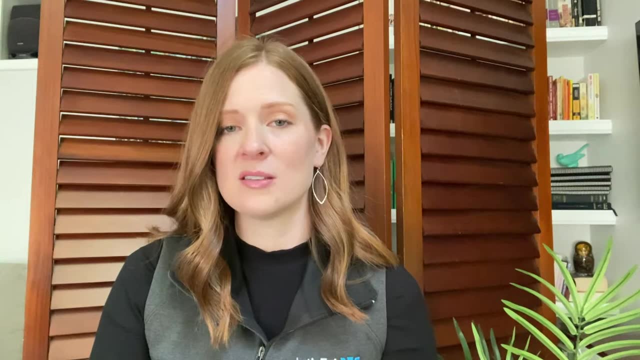 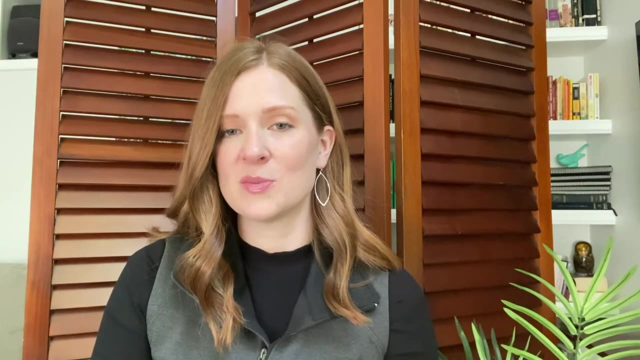 learn to interact with others, set and achieve goals and regulate their emotions. The five core pillars of SEL are self-awareness, self-management, social awareness, relationship skills and responsible decision-making. All five pillars are important for success in school. 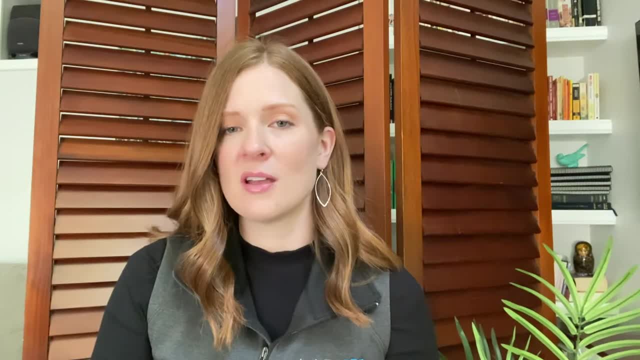 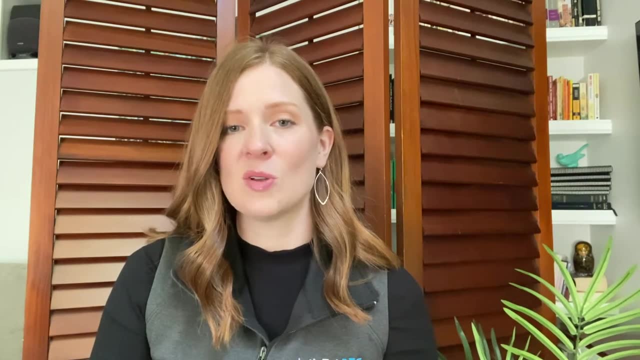 work and life. Many schools are focusing on SEL as an essential part of education to improve school climate, academic achievement and student well-being, and nutrition education can help. Nutrition education is a practical and engaging way for students to develop SEL skills. It. 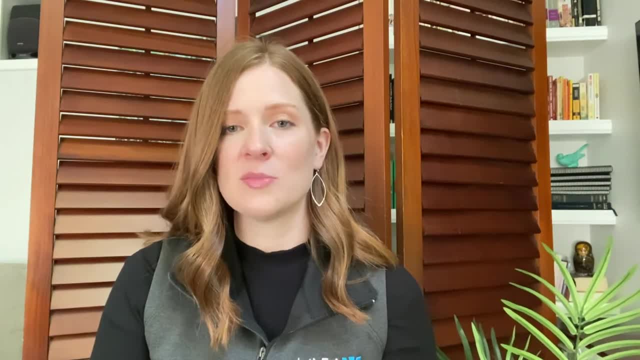 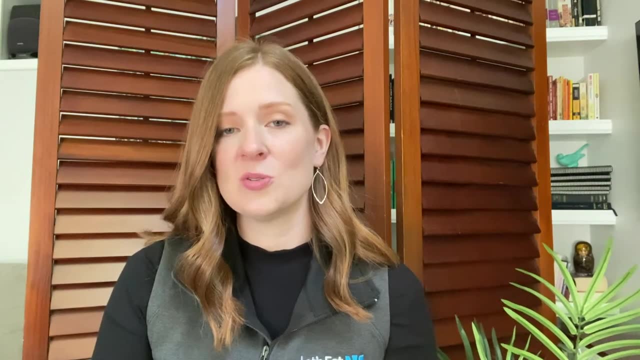 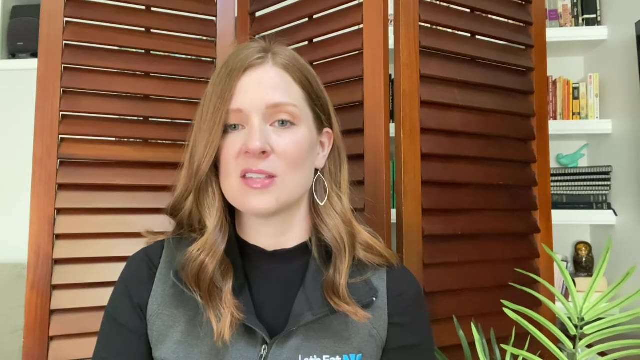 helps children practice applied knowledge skills by encouraging them to relate food and nutrition to their own health, culture and personal experiences. Teaching nutrition lessons and then engaging students in conversation about food enables them to actively practice SEL skills that will help them throughout life. Here are a few examples. 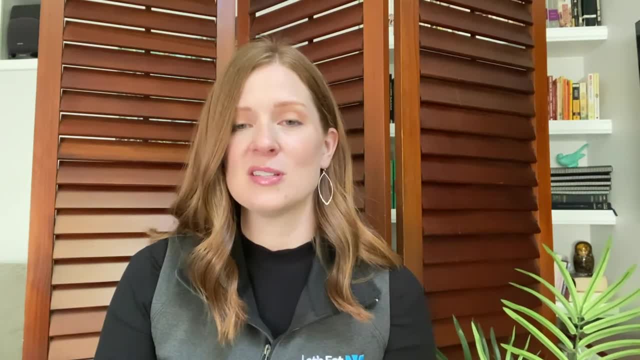 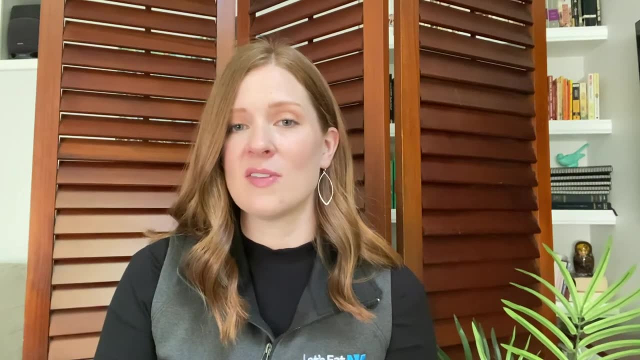 Of how nutrition lessons and activities encourage students to practice the five pillars of SEL. Food tasting activities and school gardens give kids a chance to explore foods with all of their senses, helping to build self-awareness, Educating students to pause before taking a bite and slow down while eating. 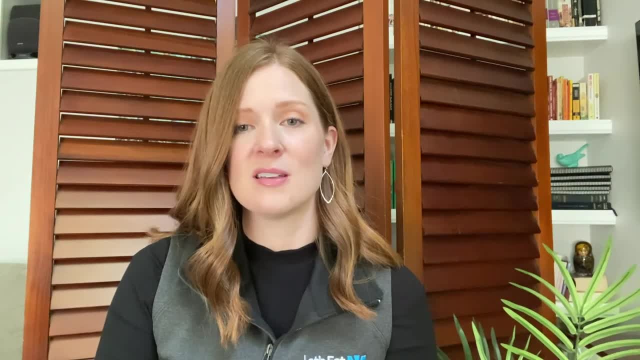 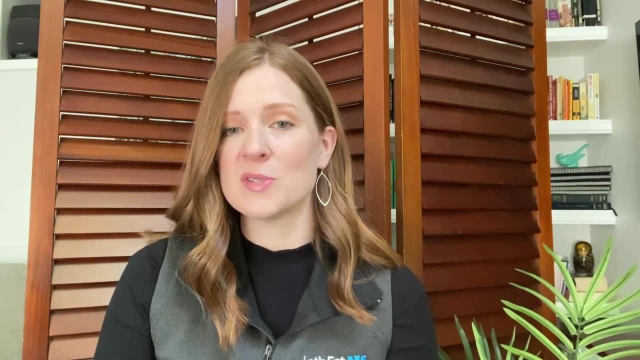 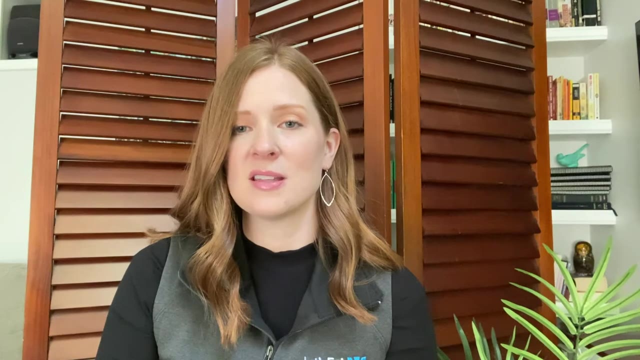 help students develop skills to manage impulse choices, set goals and practice self-management. Teaching students about where food comes from and the work it takes to bring food to our plates builds social awareness, understanding and gratitude for farmers and processes that allow us to have nutritious food. 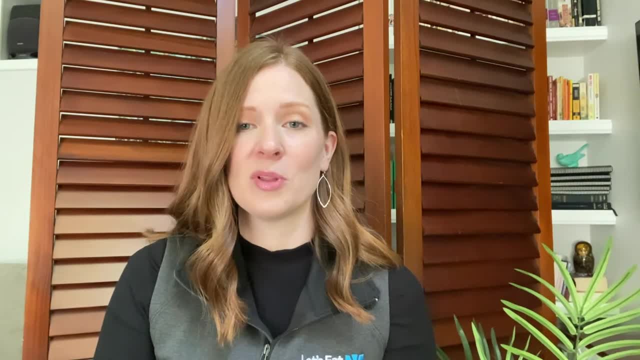 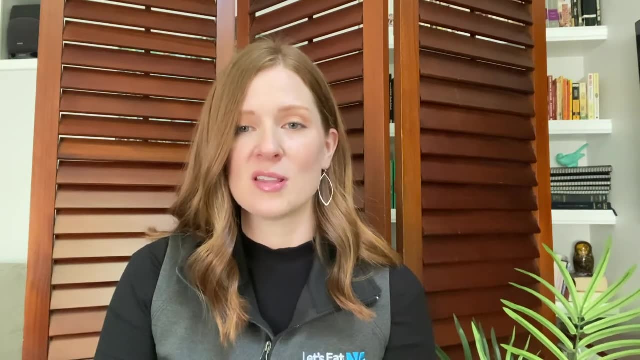 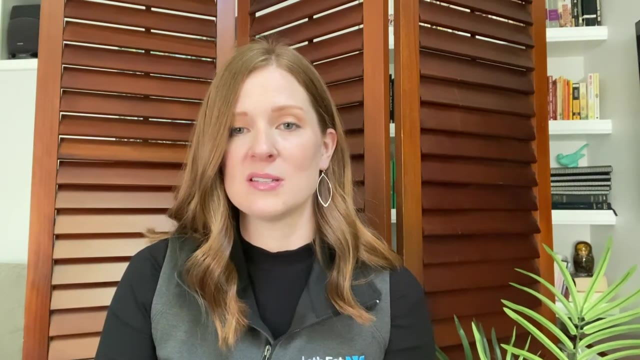 Giving students nutrition activities to complete at home and encouraging them to help with grocery shopping. menu planning and meal preparation builds knowledge and strengthens relationship skills. And, finally, nutrition lessons empower children to make healthy food choices, making it possible for them to practice responsible decision-making for their own health and well-being. 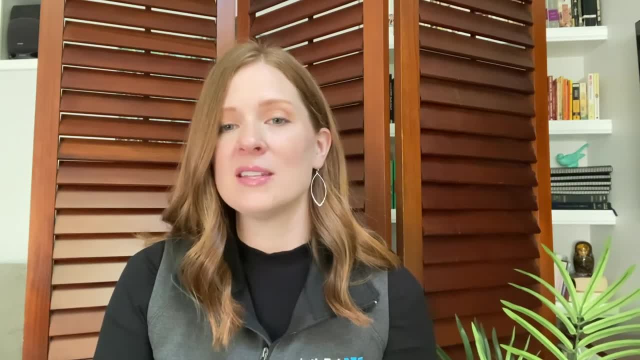 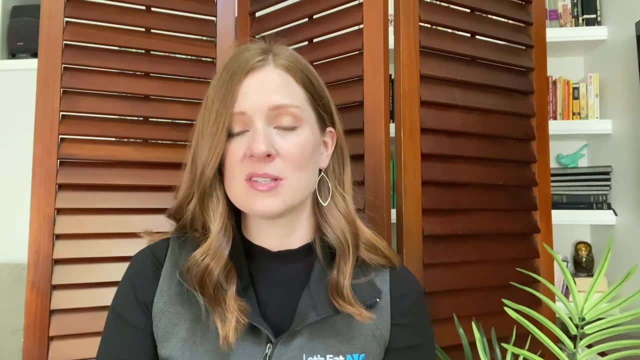 Food is a universal topic that invites kids to practice behaviors that show respect, appreciation and inclusivity of other cultures, backgrounds, languages and experiences. Teaching nutrition in the classroom is a great way for children to develop social, emotional and emotional skills.